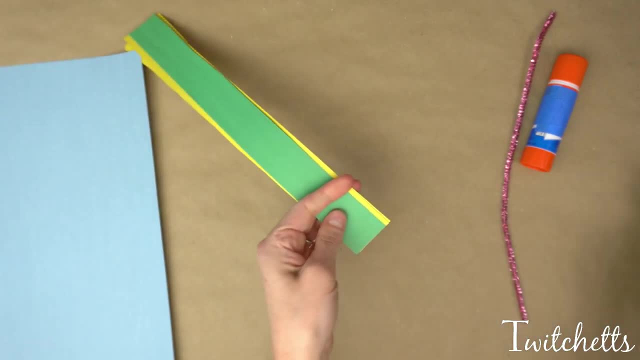 use the hole punch. they might not be able to get through all of them at once, but we're just going to do them all at one time here. Split them into groups. they can go in as far as the punch will. let them go about in the middle, if you can, and go ahead and punch. 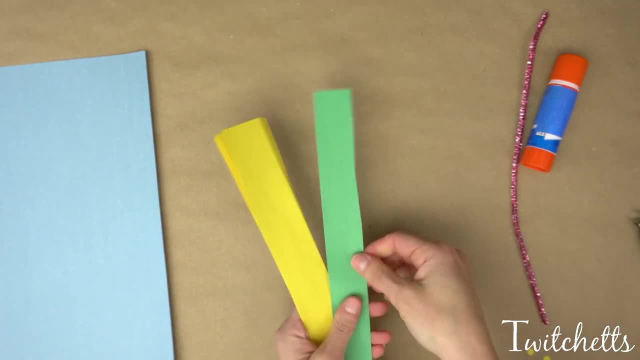 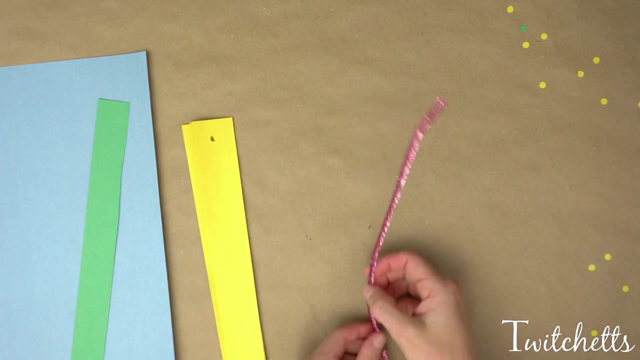 those holes out. Now the green. we don't need both sides, so take that one out of the way and then go ahead and punch the other side of your flower petal color. We'll brush those dots out of the way here. Now we're going to start with our pipe cleaner. You won't. 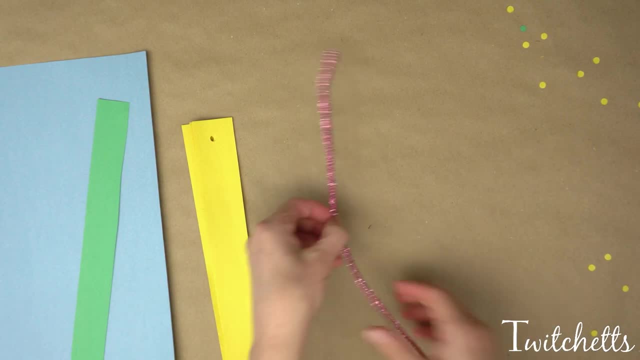 need the entire pipe cleaner, but it's going to be a little bit easier if you have a little bit of space underneath. but it's easier to work with if you've got the extra space underneath while making the flower. So go ahead and give it a good fold in the middle. 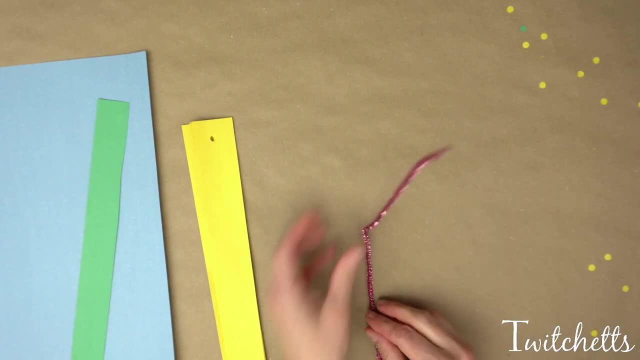 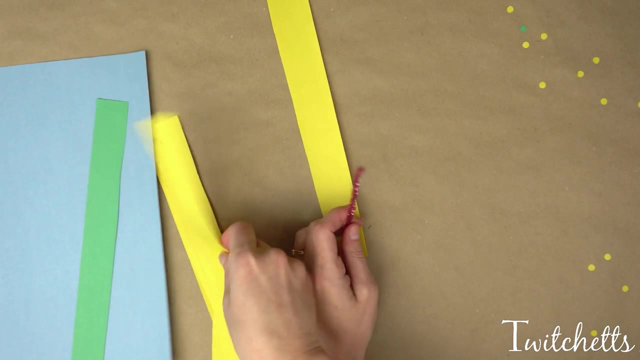 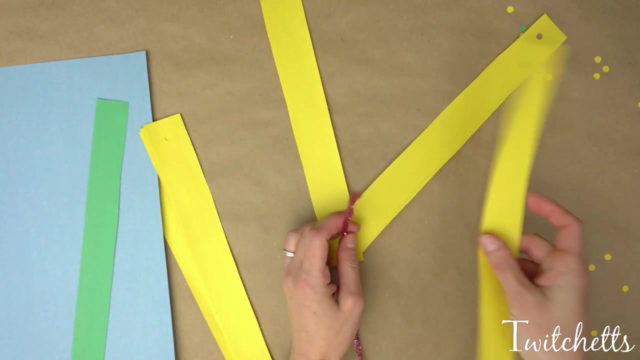 This will be our spot to basically catch all of our petals, And all you need to do is start threading your petals on one at a time, all the way around your petal. Now, if your little one is particular about their art projects, you can try to do them pencil side up and 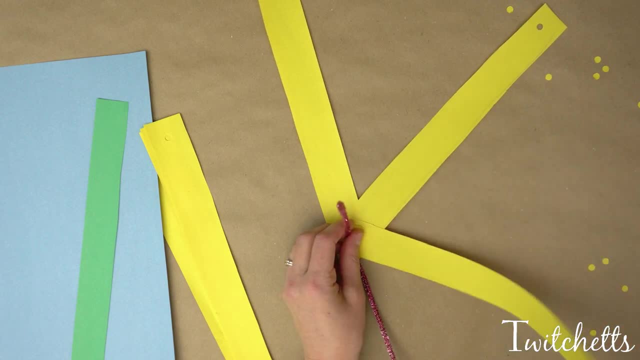 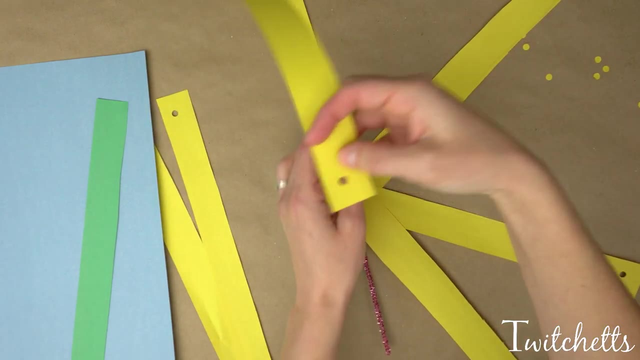 then, when we're all done, you won't see as many of the pencil lines, but I don't think it matters all that much. That's why I like to use pencil too. it's pretty light, it doesn't show up that much And, to be honest, I don't think most kids would even care, because they're. 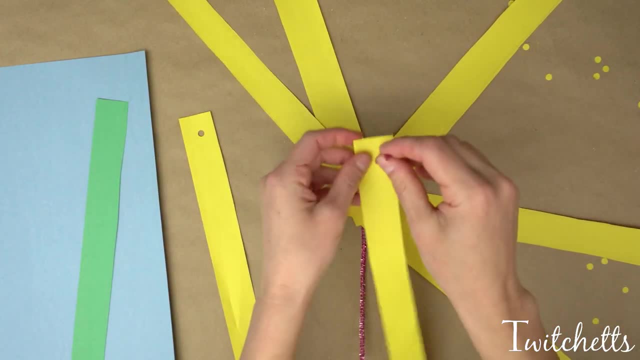 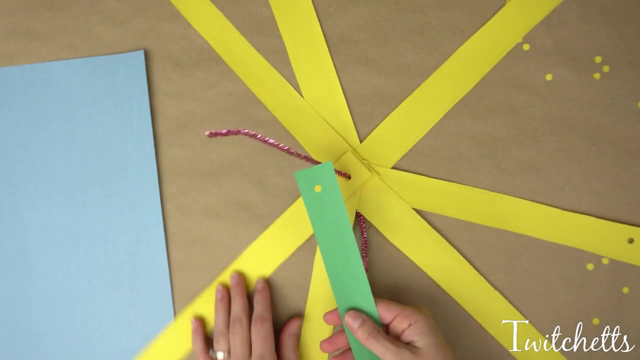 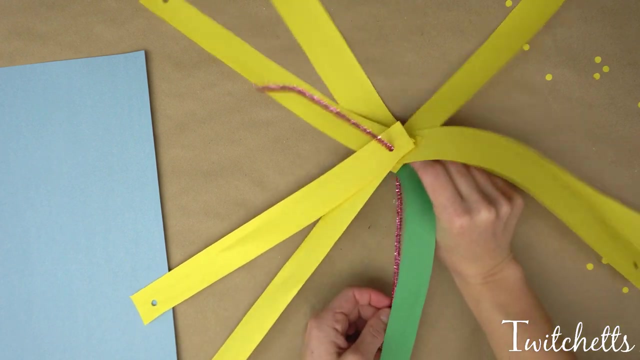 going to be so excited about their finished product, Just like this all the way around. Oh, and I forgot to put my stem on first. If you do like I do, you can always go in from the other edge And get that stem at the very bottom, like that, Or you can put your stem on first Once. 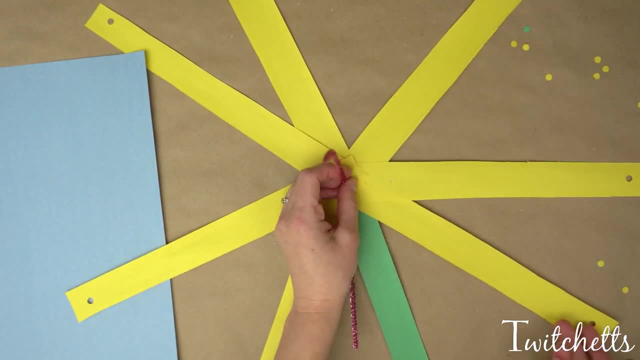 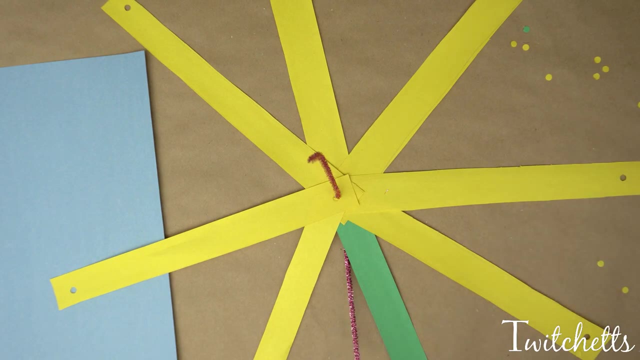 you've made it all the way around your flower, one at a time. you're going to bring your petals back to the center, But before we do that, we're going to just put down a little bit of glue, And it doesn't have to be a lot, it's just going to help everything kind of. 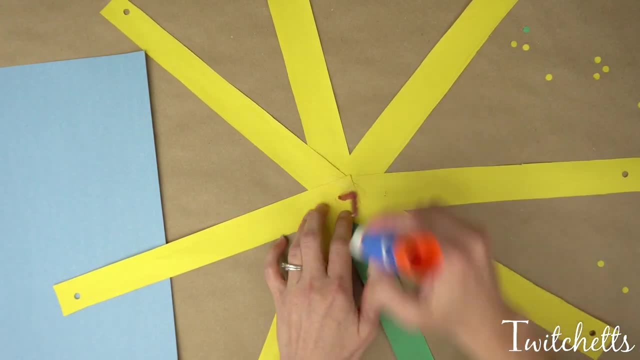 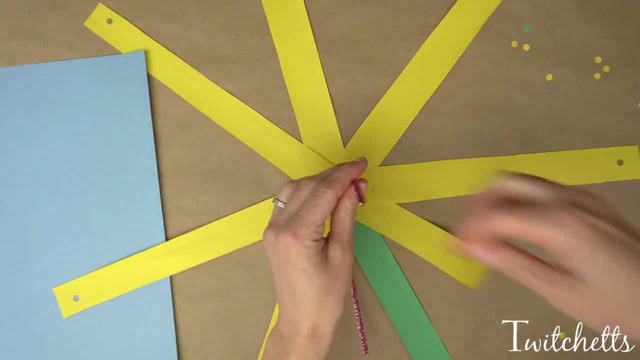 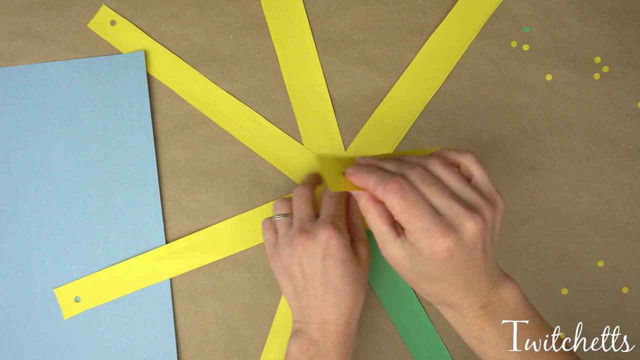 stick together at the end. So I just kind of work my way around the center here just to add a little bit of glue to the center And then, one petal at a time, we're just going to fold to the center And press all the way down And just work your way all the way. 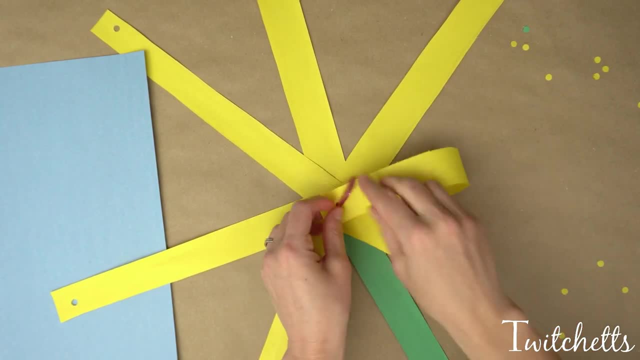 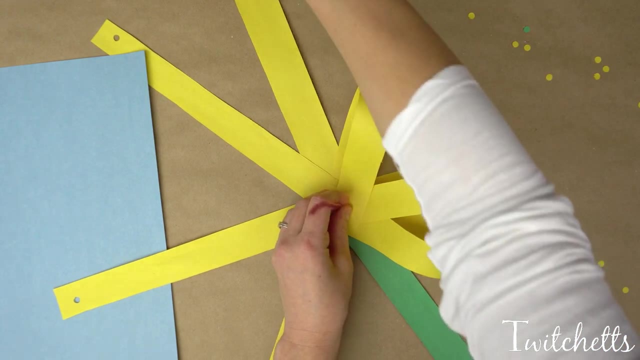 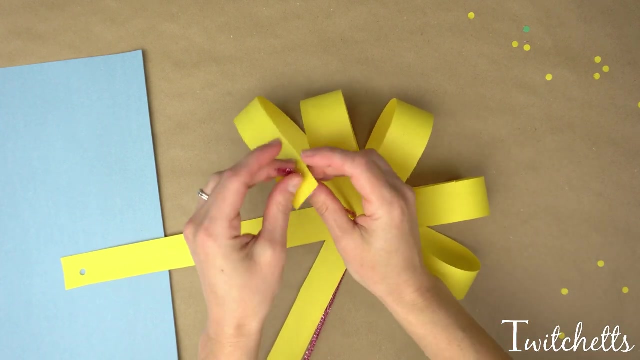 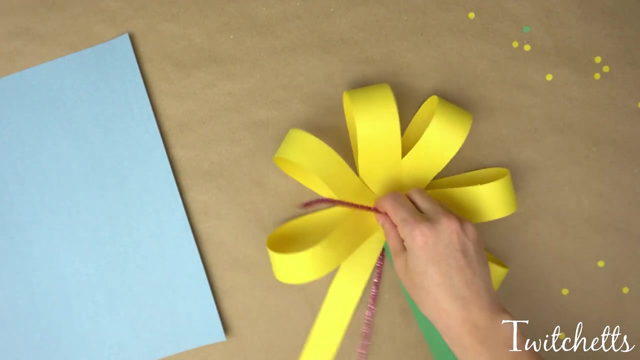 around And it starts looking like a flower pretty quick, Like this- And this is actually great for their hand-eye coordination and fine motor skills as well: Threading these pieces of paper And last one here, Just like that. Now, once you've got all the petals on, you can kind. 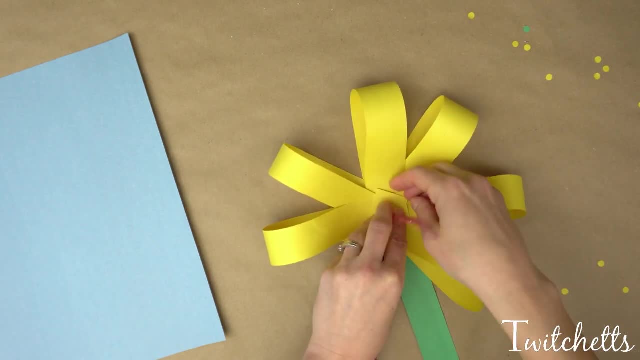 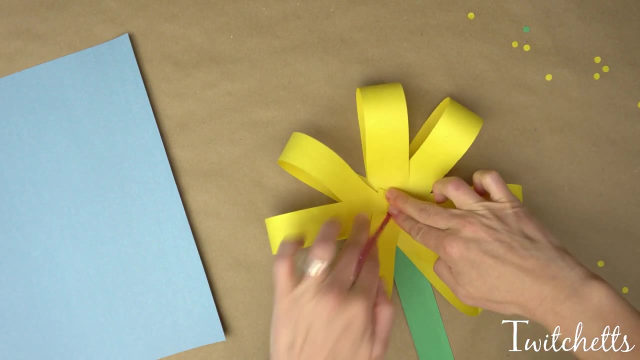 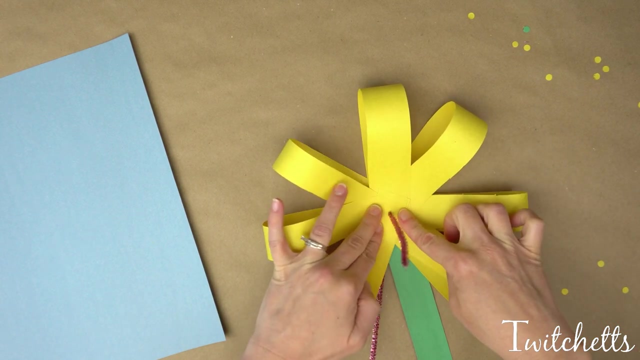 of adjust them a little bit. Once you like the shape, I like to peel up just that top petal and add a little bit of glue underneath And give it a little bit of a press down And it just kind of helps hold everything together. Now this next step might be a little 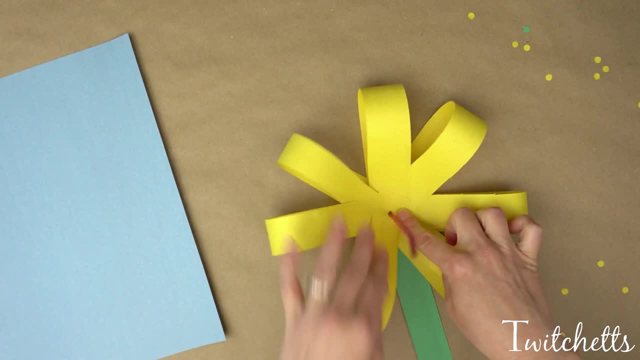 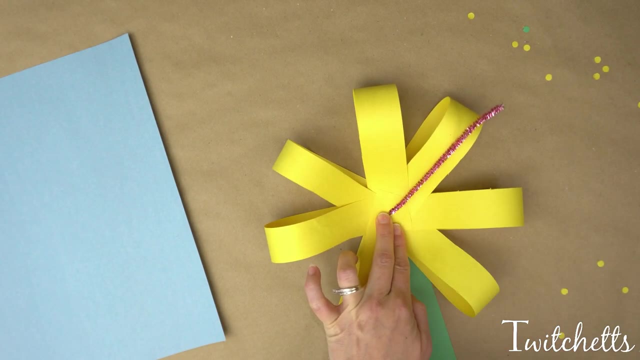 bit tricky for your younger kids, So you might want to help them with this one. What we're going to do is take our pipe cleaner and we're going to fold it to one direction or the other, And that kind of will help hold it all together when we secure the other side. And then you're 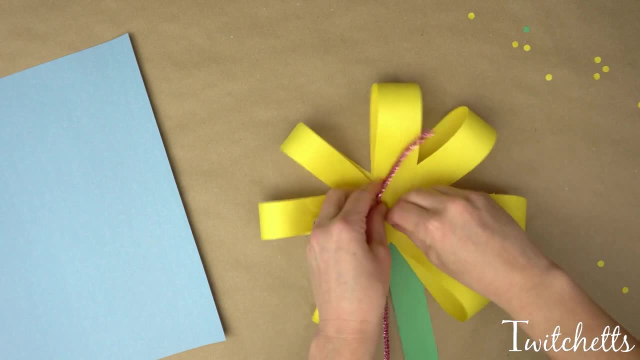 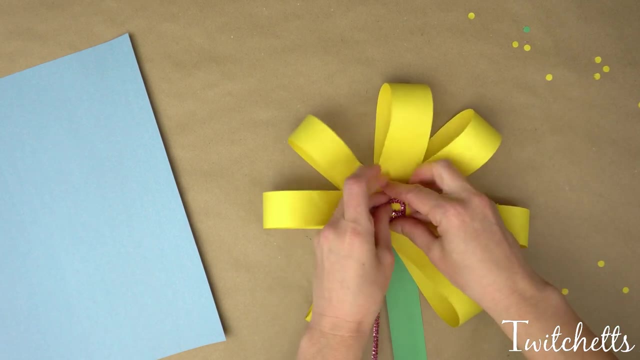 just going to kind of spin it around to create a circle in the center of your flower. So if you have really little ones, this one might be a little bit tricky. this part They can kind of bunch it up or scrunch it up as well. It doesn't have to have to be a perfect circle. 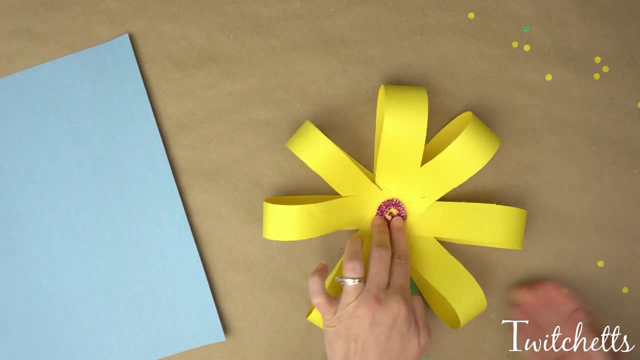 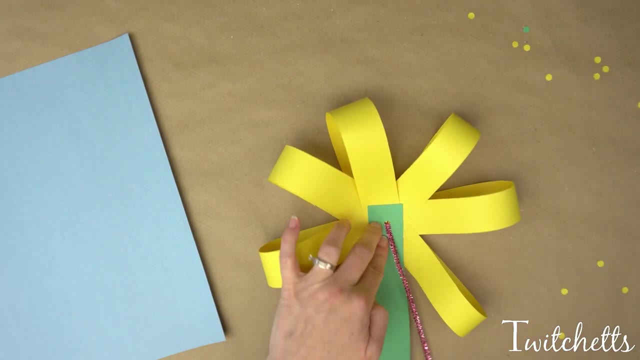 just adds a little bit of shimmer and just kind of flatten it down. and while you're holding that there, we're going to flip over our flower to our back side and we're going to do almost the same thing on the back, except it doesn't have to look pretty. we're going to just kind of zigzag. 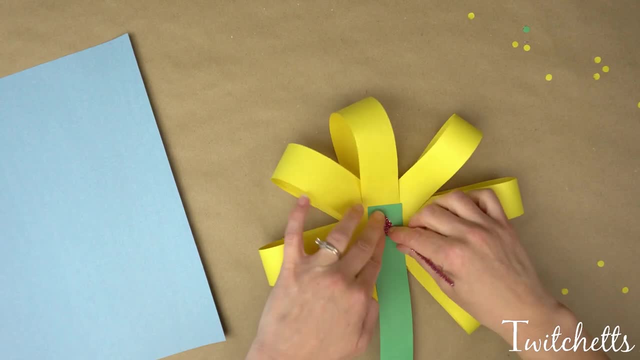 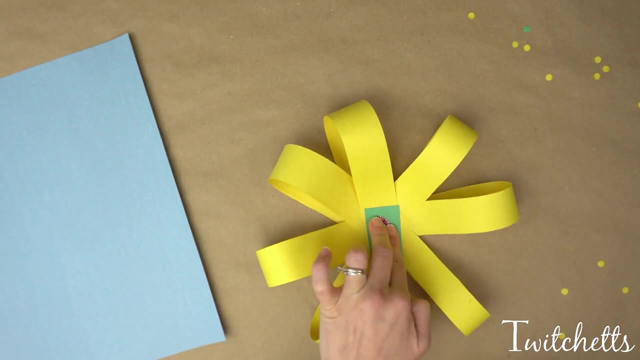 and press it down and the pipe cleaner will kind of help our flower hold together and you can go ahead and cut off a little bit of that extra. you don't need all of that on the back side of your flower and it will pop up a little bit. we want it to have that fun 3d effect. so now you need. 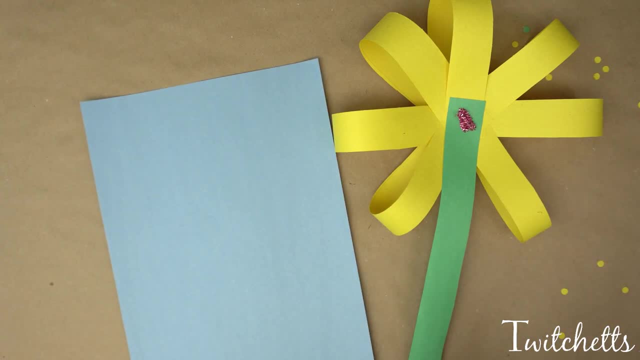 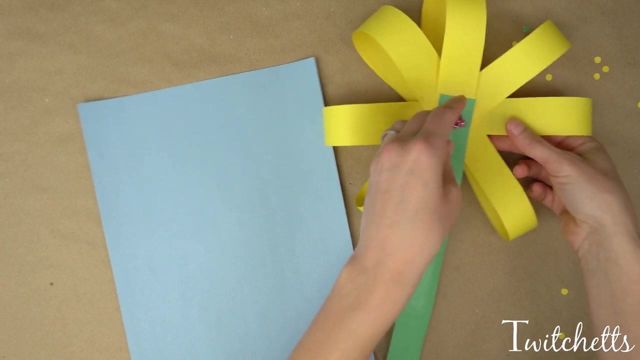 your background piece of paper and we're going to go down most of our stem. we're going to leave a little bit to fold back to be our petal at the bottom. so just give a good strip of glue here on the back of part of your stem and then we're going to flip it over onto our blue paper and you.